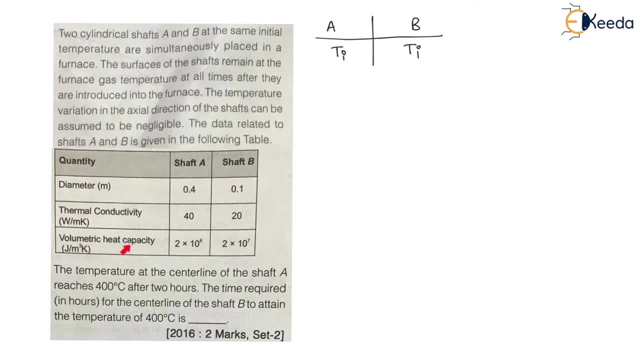 Now: quantity diameter, thermal conductivity, volumetric heat capacity. Volumetric heat capacity is nothing but product of density and specific heat. It is a product of density and specific heat. You can check the unit: Joule per meter cube kelvin. 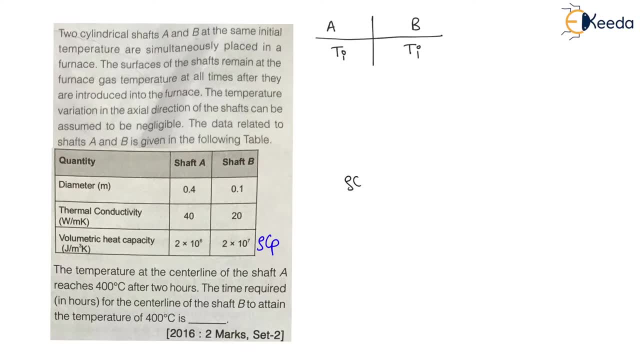 Now the volumetric heat capacity is nothing but rho, Cp. Rho is nothing but density, kg per meter cube, Cp is it is joule per kg kelvin. Therefore, kg kg will get cancelled. The unit will become joule per meter cube kelvin. 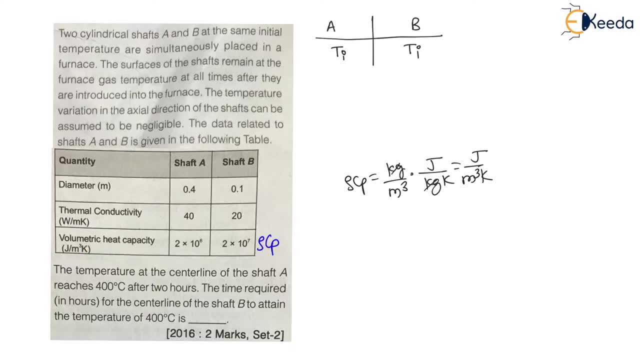 Right, This is called volumetric heat capacity. Therefore, it is a product of density and specific heat. Right Now here, thermal conductivity K is given, diameter D is given. Therefore, I will write: it is a diameter D, It is thermal conductivity K and it is a rho Cp. 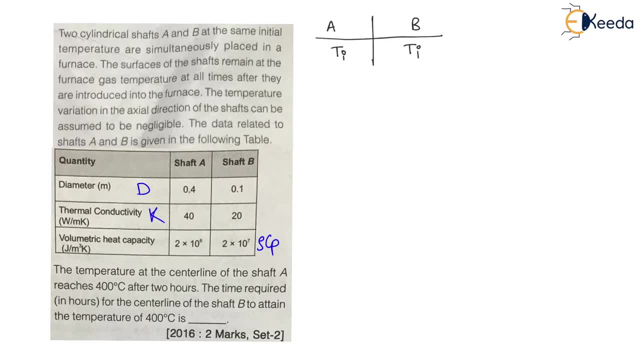 Right. Therefore, let us write here, Let us write down data. Therefore, the diameter of A is nothing but 0.4.. Diameter of B is different. It is 0.1 and it is in meter Right Thermal conductivity K. it is in watt per meter kelvin. 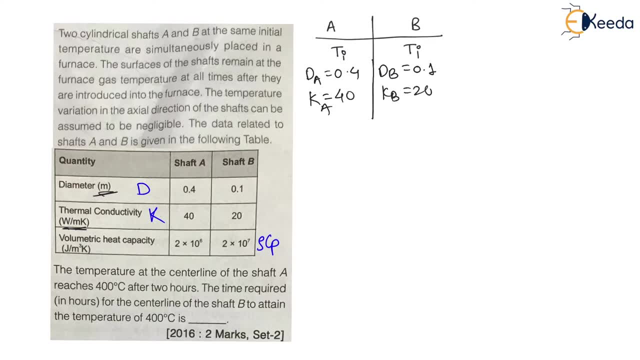 40 for A and thermal conductivity of B is 20. Then rho Cp of A will be 2 into 10 to the power 6. And rho Cp of B will be equal to 2 into 10 to the power 7.. 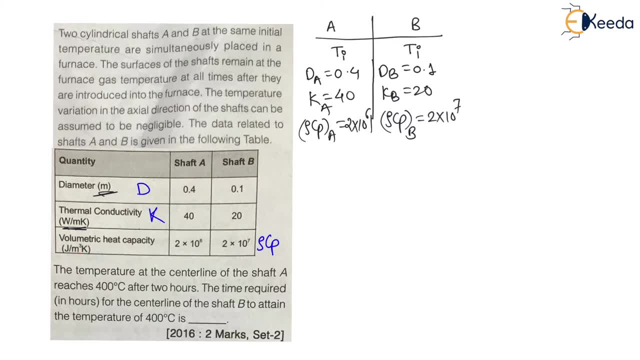 It is joule per meter cube kelvin Here. I am not writing unit because all are standard units Right Now. then question is: Temperature at the center line of the shaft. A reaches 400 degree Celsius after 2 hours. Now. here time is given. 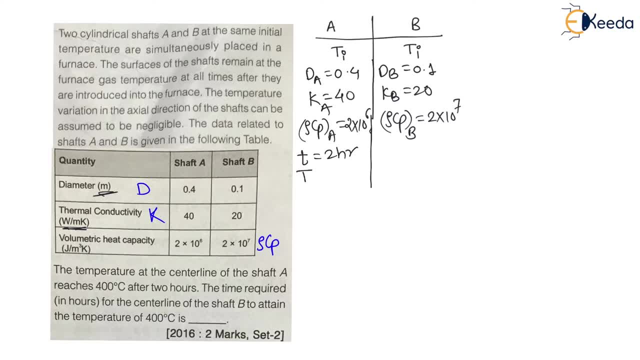 Time T is 2 hour. After 2 hour, the temperature of center line of shaft A reaches 400 degree Celsius. Let us say this temperature as. Let us say this temperature as T. Right Then the time required in hours for the center line of shaft B to attain the temperature. 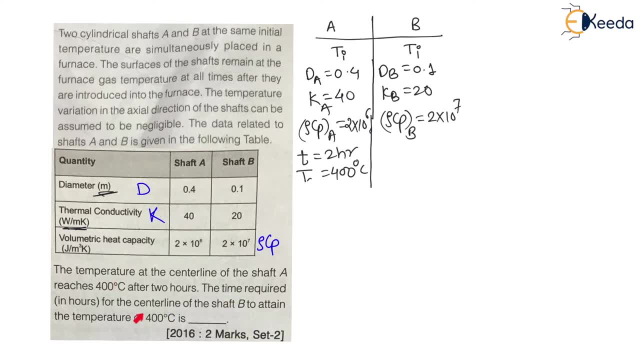 of 400 degree Celsius. Again for B, the same center line temperature. Therefore, again here, what will be the time for B? Time for A is 2 hour. Time for B is equal to question mark in hours. We have to find in hours. 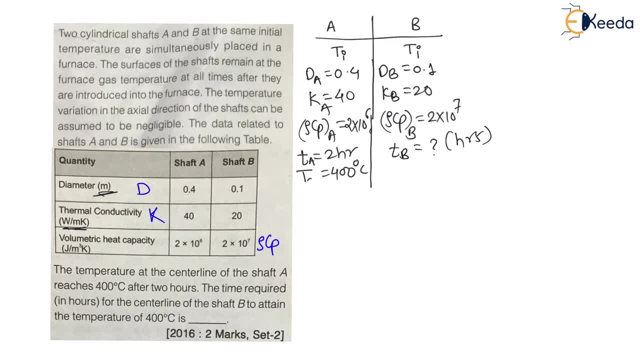 Right, Then in question mark whenever the temperature is again 400 degree Celsius. Right Now, my dear students, We have one formula: that Temperature minus initial temperature divided by surrounding temperature minus initial temperature is equal to error function. T, Right, Z, x, f. 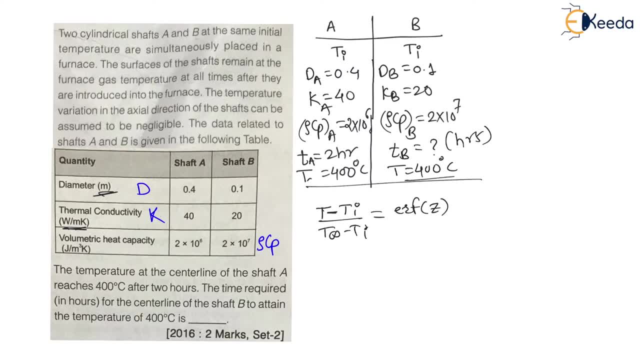 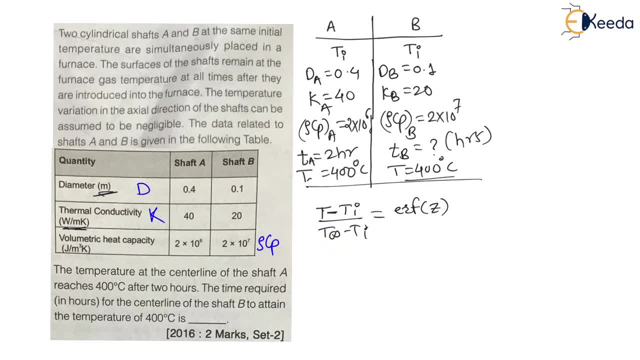 Right Now, here, temperature for both is same. Initial temperature is also same, Surrounding is same, The same surrounding is there means surrounding flow temperature is also same, That is P. infinity is same, Right. Therefore, my dear students, can I say this error: function Z will be same for both. therefore, 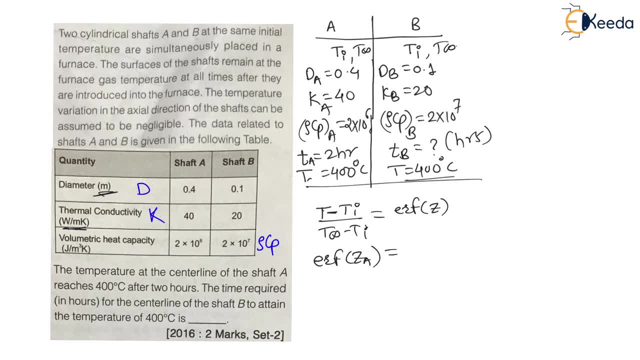 I can say: the error function Z of A will be equal to error function will be equal to error function z of b. therefore, can i say this: z a is equal to z b. z a is equal to z b. right now. with the help of this now simple calculation. now it is very simple. 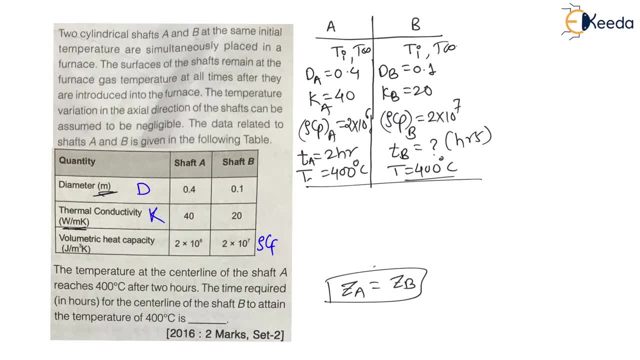 calculation. now, here we have seen. error function is same in both cases. now what is the formula of this error function? if you remember carefully my lectures, then this error function is nothing but error function. of this error function is nothing but radio, because heat transfer is along radial. 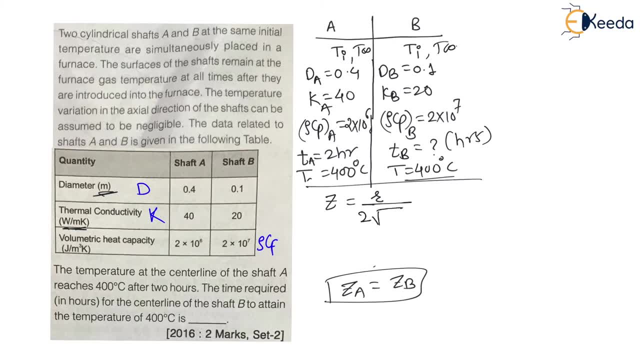 direction. divided by 2, under root of alpha time, t. right here, alpha is nothing but thermal diffusivity. this alpha is thermal diffusivity, t is the time and r is the radius. right now, this is the error function. therefore, my dear students, here can i write error: function of a is equal. 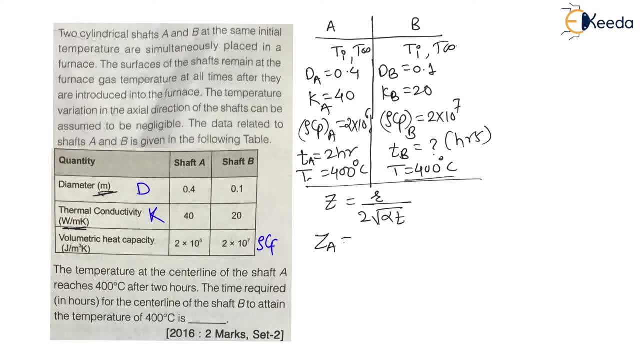 to error function of b. right here we have seen: z a is equal to z b. therefore r, they have a, 2 under root of alpha a. ea will be equal to rb. they have a, 2 under root of alpha b- eb. right now, with the help of this calculation we will definitely find, or easily find, 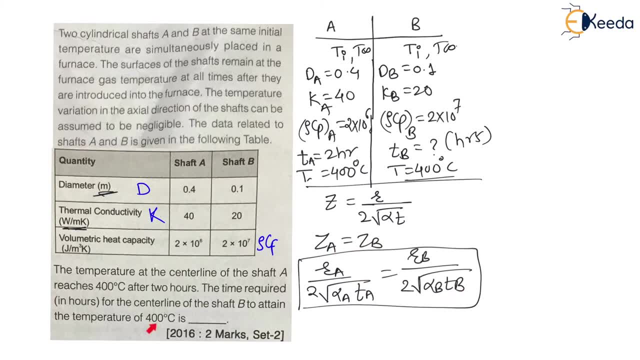 this time of b, time required for b to reach centerline temperature of 400 degrees celsius. now, my dear students here, alpha, alpha is thermal diffusivity, that is, it is a ratio of thermal conductivity and volumetric heat capacity. right, we can say this: alpha is nothing but thermal. 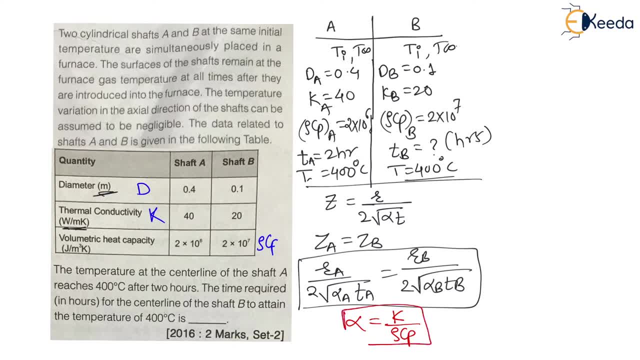 conductivity divided by volumetric heat capacity, k divided by rho cp is called thermal diffusivity. so here k values are given this, volumetric heat capacity values are given, that is rho cp. so let us put these values right now. my dear students, write down this quickly because i am 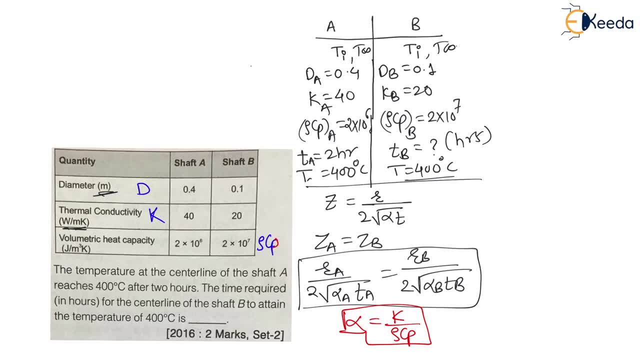 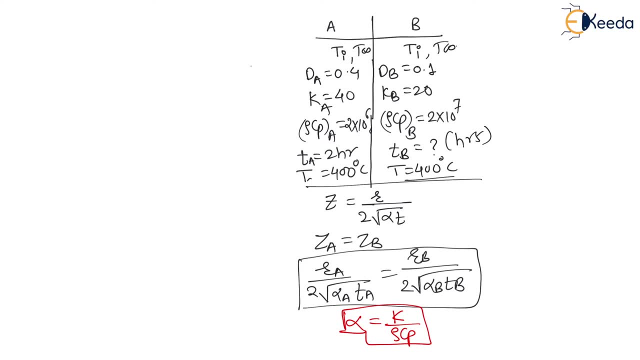 going to erase this question. now, let us delete this question. if i delete this question, i will get space now here. therefore, let us equate this error function. therefore, my dear students, can i say here: 2, 2 will get cancelled from both sides. now here. radius: radius of a is: 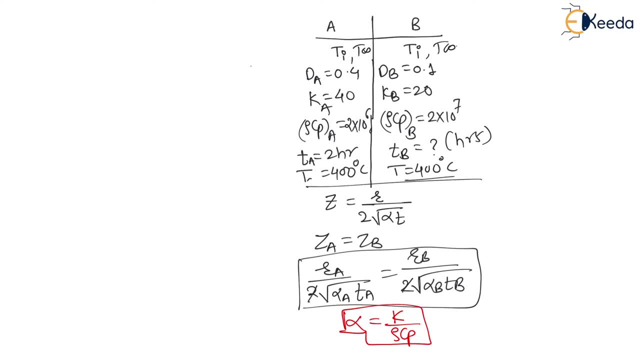 nothing but diameter divided by 2. right, therefore? here let us write: radius of a divided by under root of alpha a is nothing but k divided by rho cp of a into time of a is equal to radius a divided by rho cp of b into time of b. now let us square both side. if i square, then i will get. 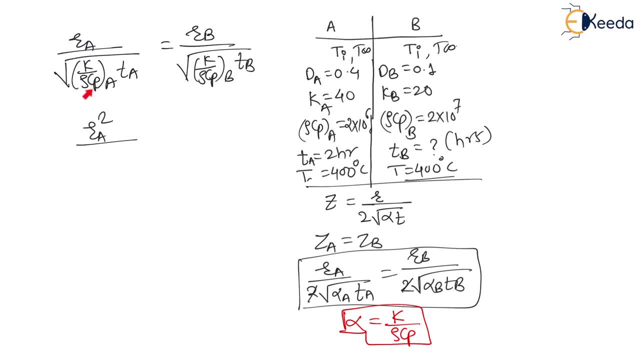 r a square divided by now. this rho cp will go up into rho cp of a whole divided by k of a time of a will be equal to r b square divided by. again, this rho cp will go up rho cp of b divided by k of b. 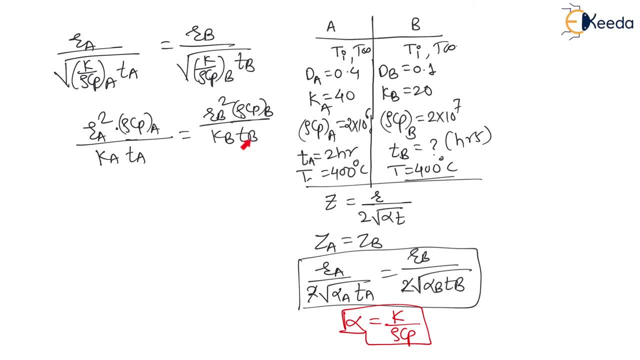 time of b right now. let us find this time of b. so if i want to find this time of b, therefore time of b we will get is equal to. it is nothing but r b square into rho, cp of b into k a. p a divided by r. 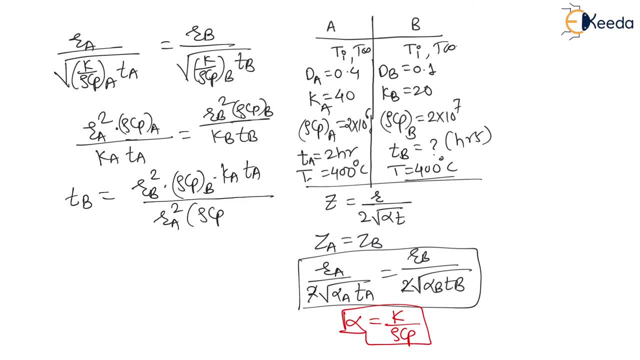 a square, into rho, cp of a, into this k of b, k of b. i can write here also: k of b is in the denominator, right now, everything you have, all the values we have, so let us put the values. therefore, this time of b will be equal to now here. radius of b is, diameter of b is 0.1. therefore, we can say this: 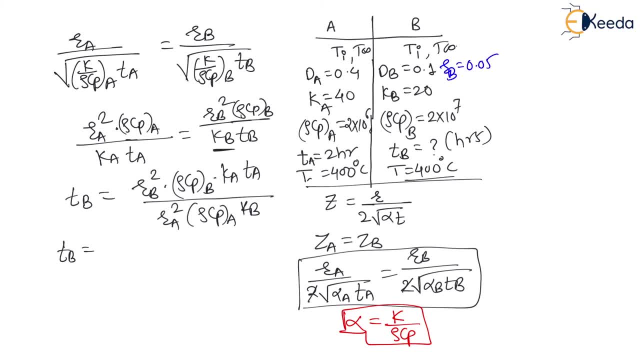 radius of b will be equal to 0.05. diameter of a is 0.4. diameter of a is 0.4. therefore, radius of a will be 0.2. so let us put these values, therefore. here, radius of b is 0.05.